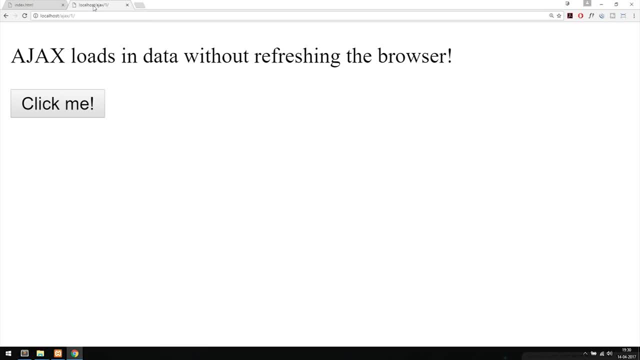 one you guys can see here and I have an identical one that is in here Now. both of these have AJAX inside of it, inside the code, but only one of these are inside a server. So this website here is just inside a root folder inside my desktop and the other one is inside a local server I installed. 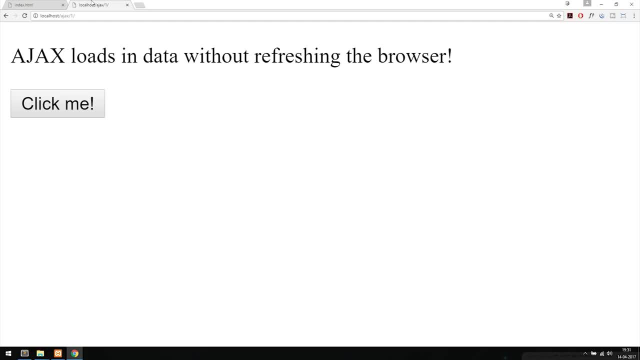 using XAMPP, and you will in fact learn how to actually install XAMPP and how to get a local server up and running. It's very easy to do, but for now I'm just going to go and show you guys what exactly AJAX can do. So inside the first tab here. I'm not inside a server, so were to actually click. 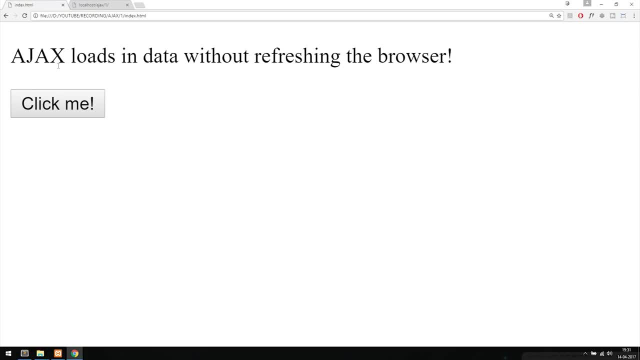 the button, nothing happens. Now, if I were to go to the second tab and click the button, you guys can see that I changed the text. So basically what I just did here is I went ahead and clicked the button and then I replaced the text with: 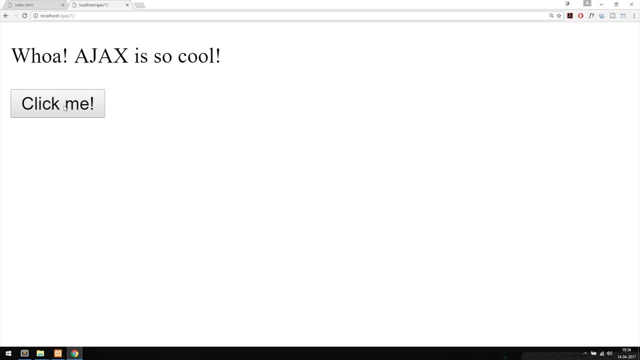 another piece of text that was inside a separate document inside my server, and I did all that without having to refresh the browser. Now, this might not seem very impressive if you're not used to PHP and handling databases, but this feature here is actually something that's really needed. 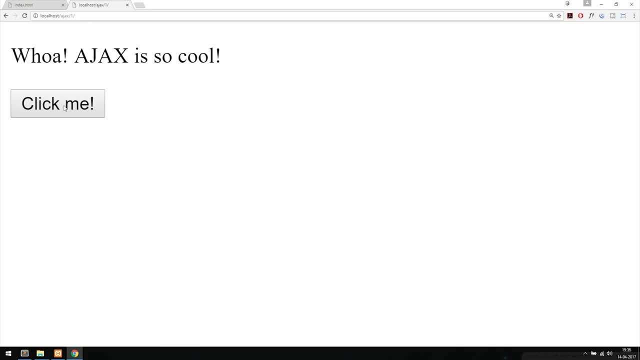 when you want to get data from a database and put it inside a website. Again, I want to mention that you don't need to know PHP or about databases in order to use AJAX. it's just something that you can use together with PHP and databases in order to get data without having to. 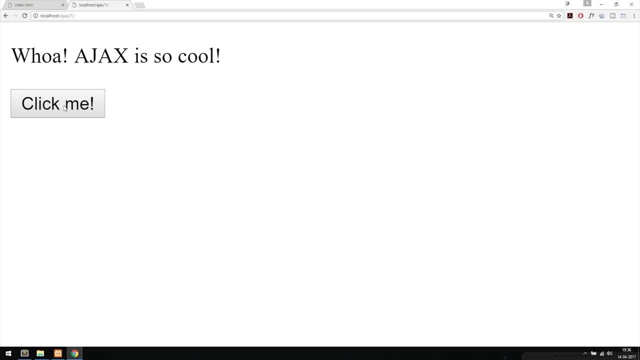 refresh the browser from a database. I'm mentioning this because I know a lot of you guys will have a PHP background and you will be using AJAX for getting data from a database, So I just want to include this. but AJAX is not only for people who want to pull in data from a database, it's also for 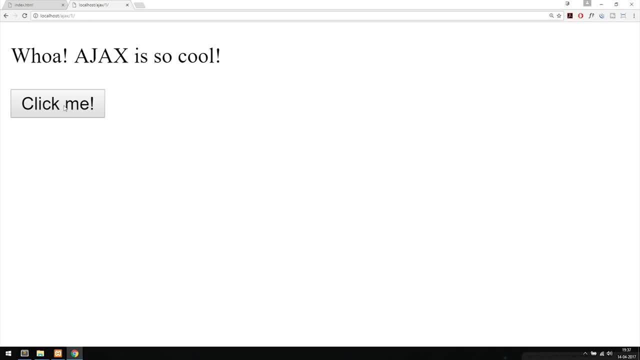 people who just want to get data from a server without having to refresh the browser. Now, when it comes to AJAX, there's actually two different types we can use. We can either use AJAX with JavaScript or jQuery. Now, because jQuery is the easiest one to learn, I'm going to go and start. 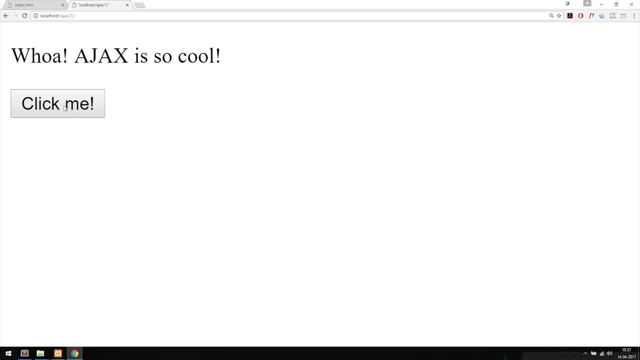 out the series by doing the jQuery way and then afterwards we're going to learn how to do it using JavaScript. So in the next episode we'll talk about how to actually do stuff using AJAX. so I hope you guys enjoyed and I'll see you guys next time.